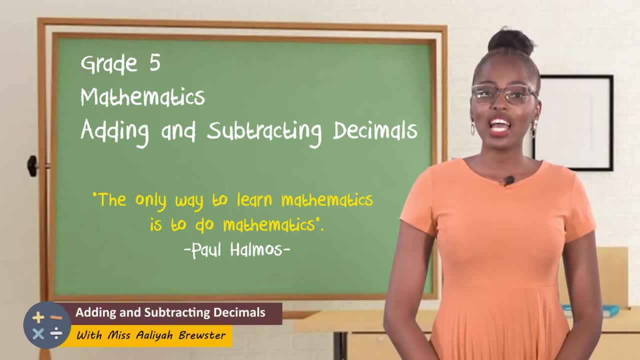 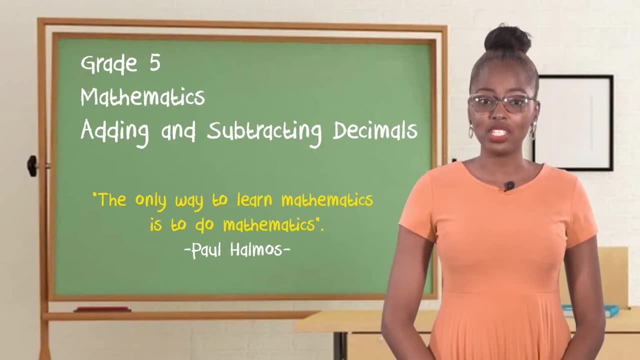 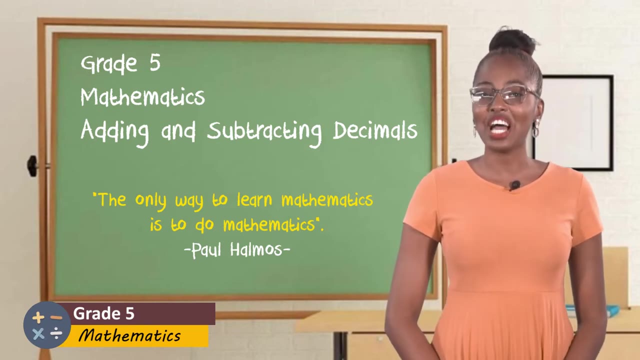 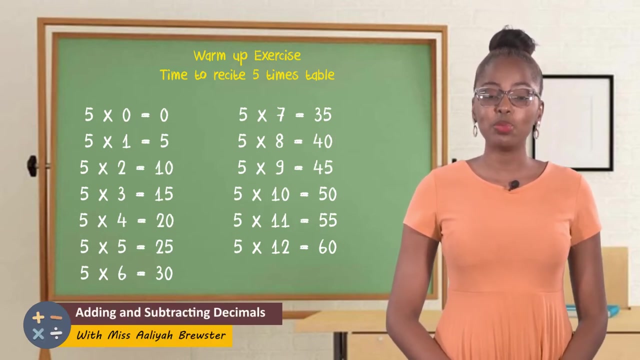 Hello boys and girls, my name is Ms. Aaliyah Brewster and today I'll be guiding you through the concept of adding and subtracting decimals for grade 5 mathematics. So grab a pencil and a notebook, get settled because we're about to start. Are you ready? Because I'm ready, let's begin. I always like to start with a warm-up exercise. So for today's exercise, we'll be reciting the 5 times table. Let's go. 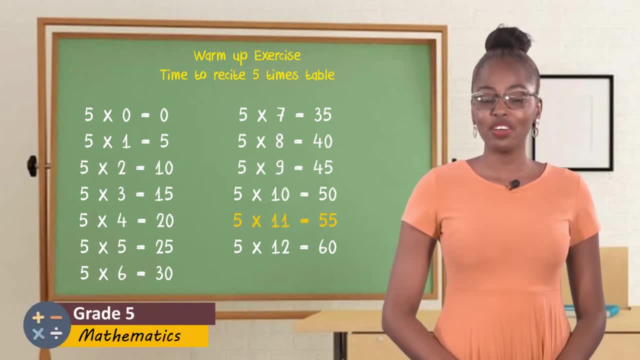 4 out of 5, 5 times 10 is 50, 5 times 11 is 55, 5 times 12 is 60. Now we'll do our questions. What is the product of 5 and 10? 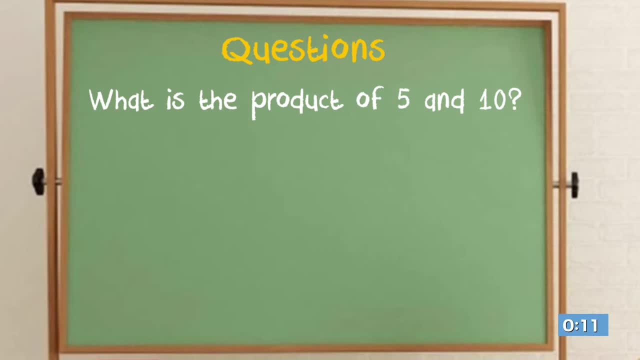 The product of 5 and 10 is 50. How many 5s are there in 20? 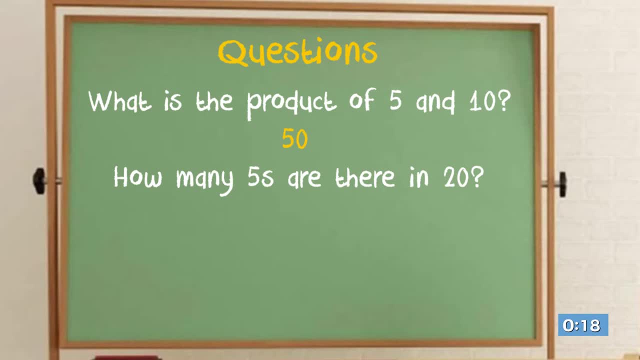 How many 5s are there in 20? There are 4 5s in 20. 5 groups of 6 is how many? 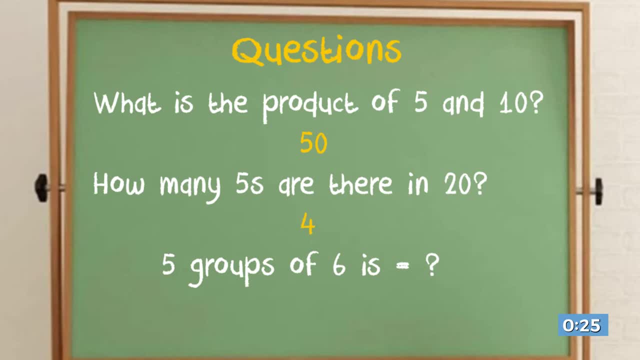 How many groups of 6 is how many? How many groups of 6 is how many? 5 groups of 6 is the number of 5s. 5 groups of 6 is how many? 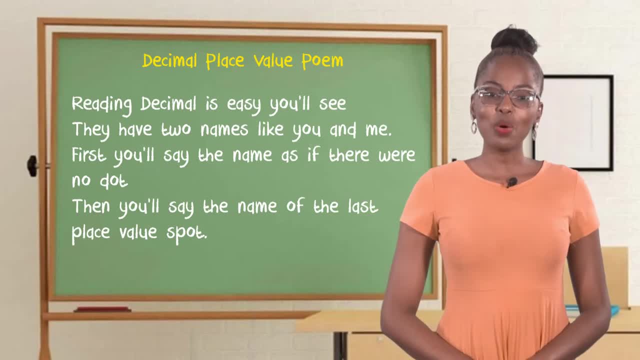 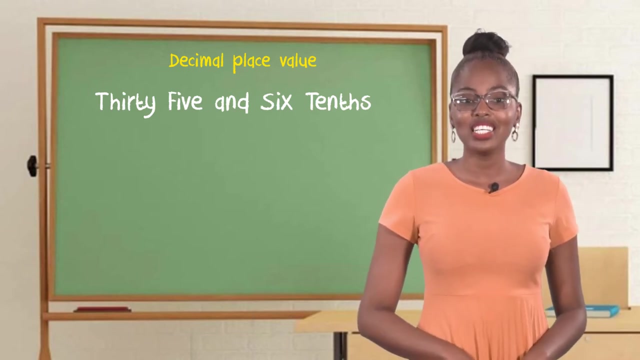 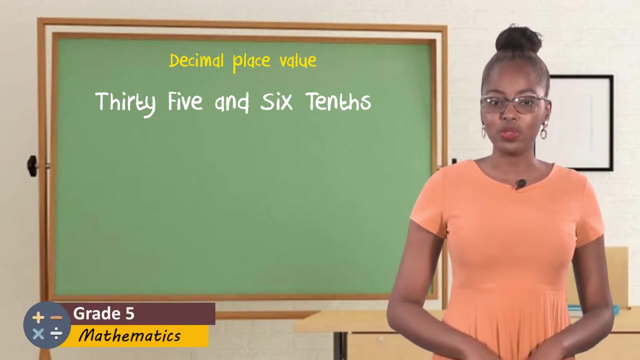 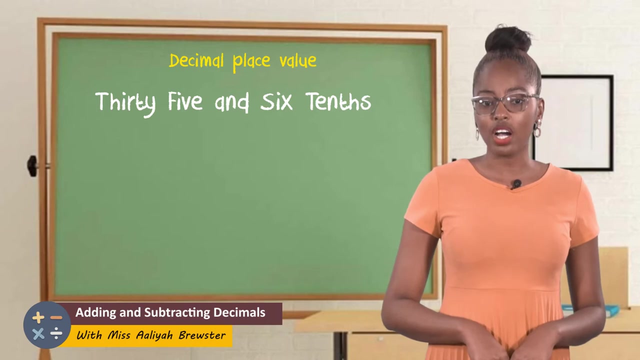 6 equals to 30. Now I'll move on to saying a poem. The name of this poem is called decimal place value. Reading decimal is easy you'll see. They have two names like you and me. First you'll say the name as if there were no dot. Then you'll say the name of the last place value spot. Place values. From the poem you'll notice that the central topic there is place value and being able to read and write place values. So let's take a step back and try to understand exactly what place values are. Now on the screen you would notice we have the number 35 and 6 tenths. 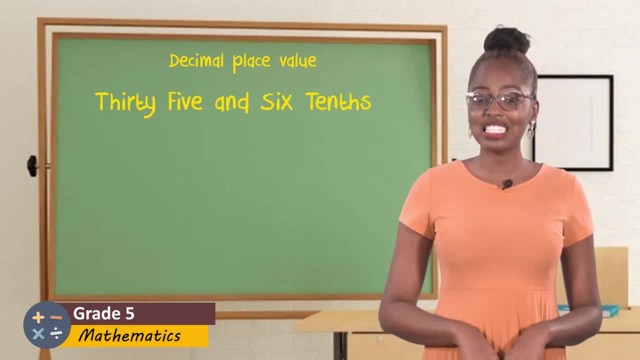 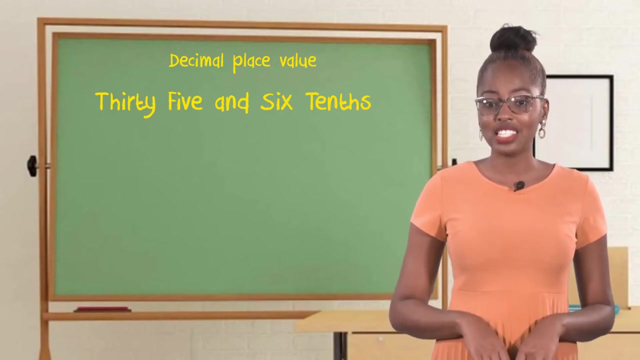 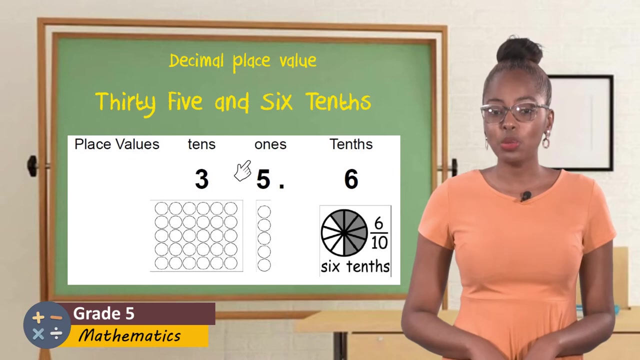 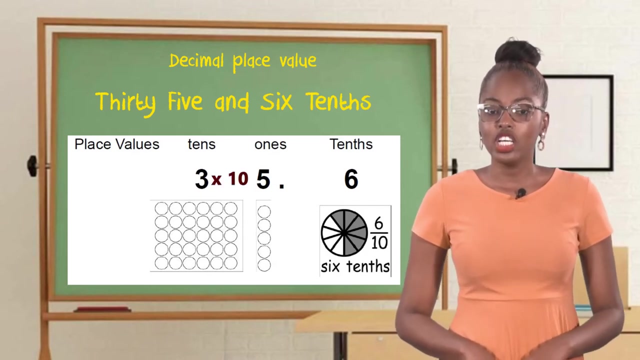 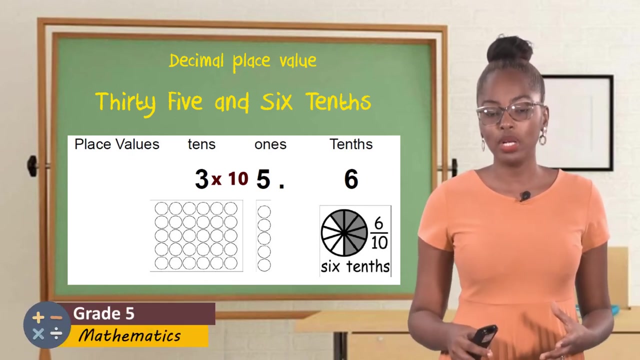 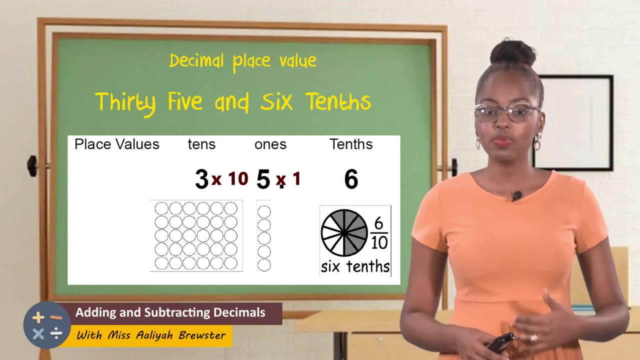 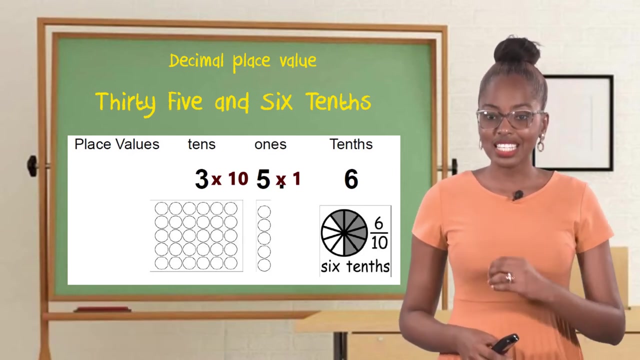 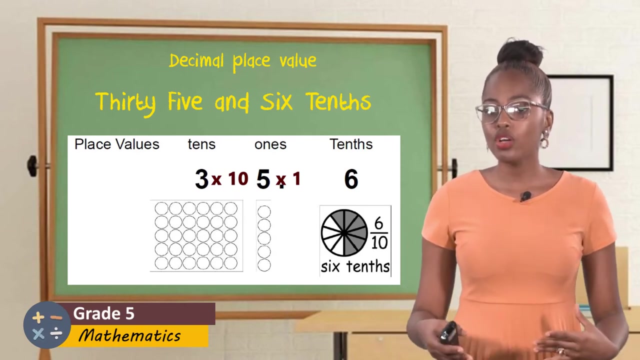 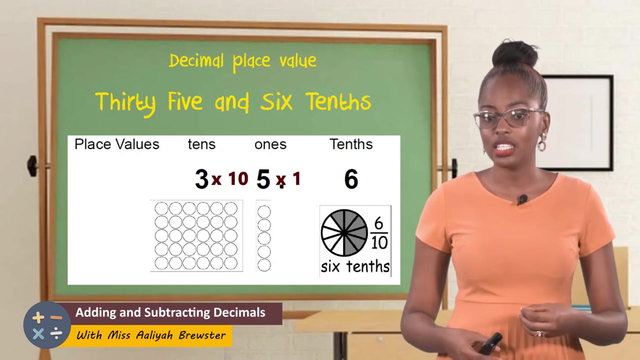 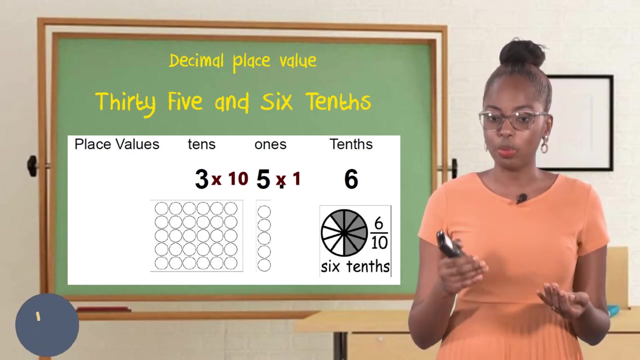 I repeat 35 and 6 tenths. I did not say 35.6. I did not say 3 5 point 6. How we say the name of this number? We say 35 and 6 tenths. The place value of 3 in this number would be tens. While the place value of 5 would be ones and the place value of 6 would be tenths. Now to break this down further, if we are saying that 3 is in the tenths place value, that simply means that 3 multiplied by 10 is an expression of the worth of that place value. So 3 there is actually worth 30, while 5 as ones is worth 5 single units or 5 ones. However, 6 tenths is represented not as a whole number, but a part of a whole. Therefore, we can represent 6 tenths with a fraction. What 6 tenths is saying is that out of a whole, that is divided into 10 pieces, 6 of those pieces are occupied. 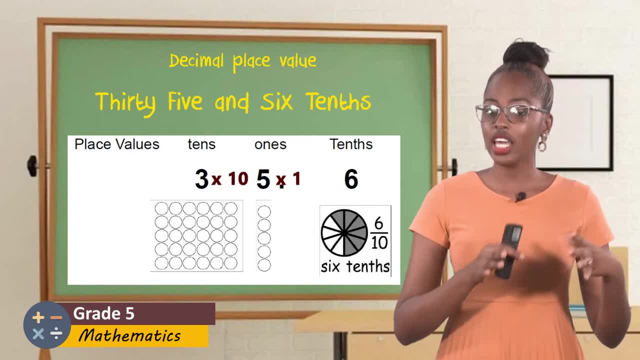 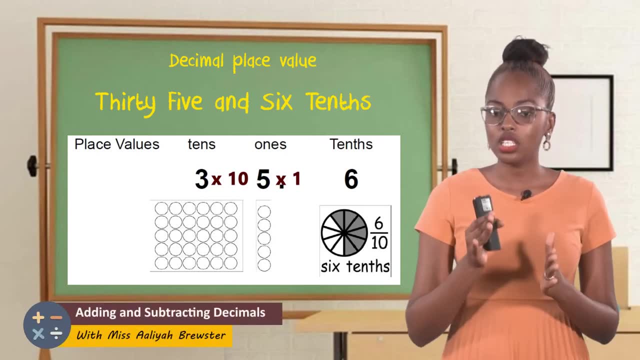 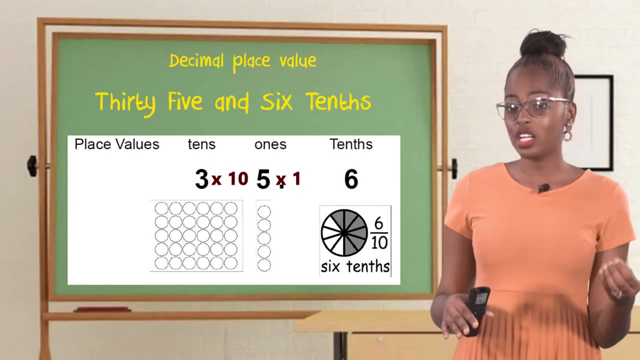 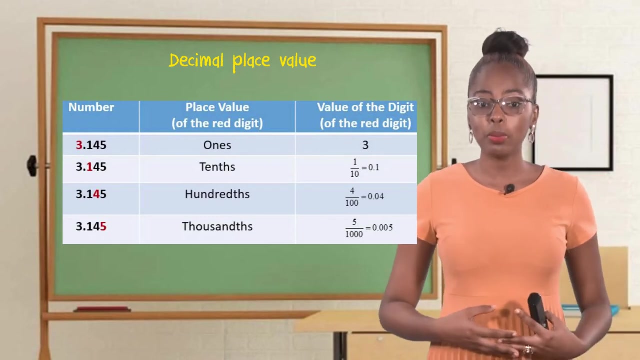 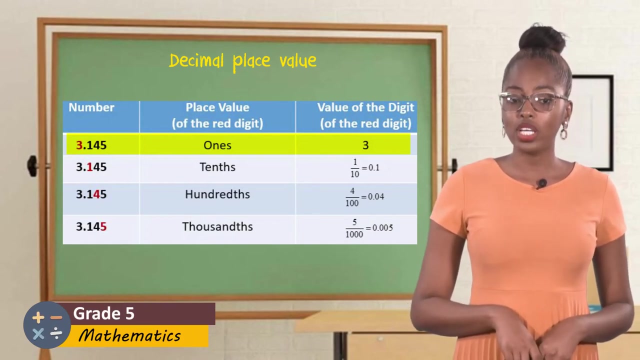 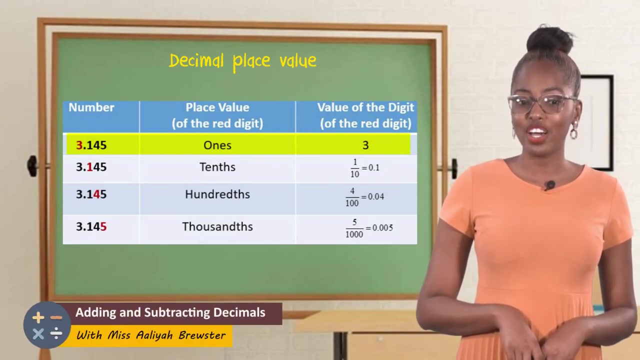 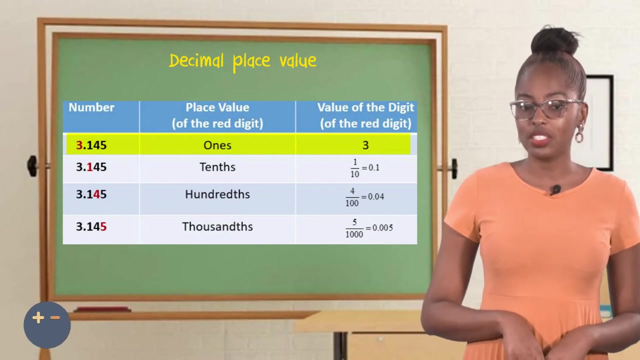 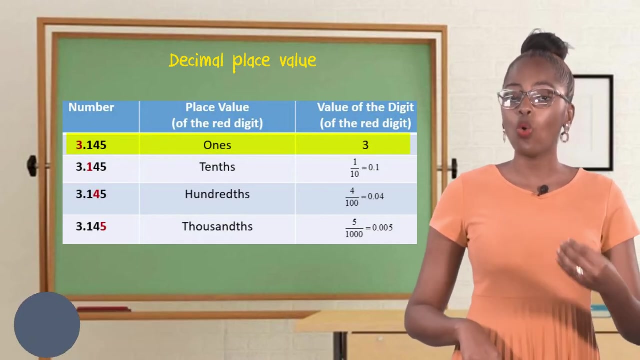 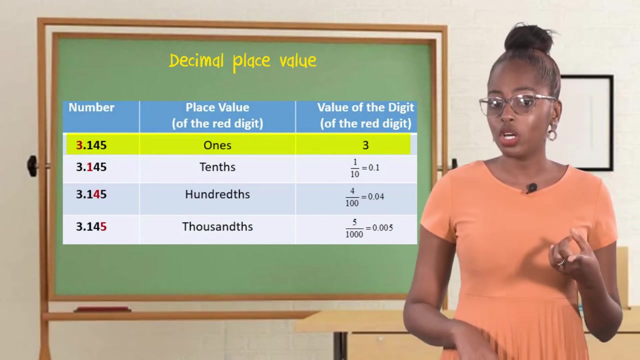 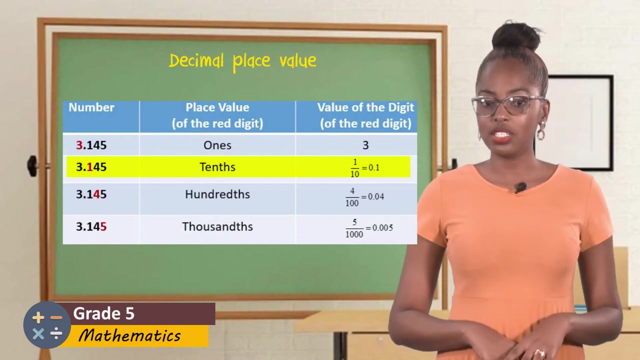 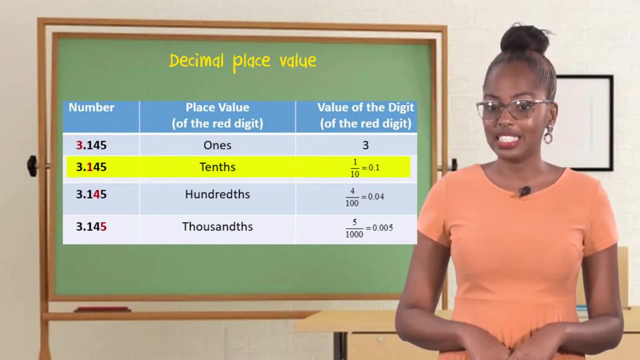 Therefore, six tenths is not a whole but in fact it is part of a whole. So it's important to note that the numbers that come after the decimal point are not whole numbers but in fact they are less than whole numbers. They are part of a whole. Here we'll develop a deeper understanding for decimal place values. For this exercise we look at the number 3.145 hundreds. 3.145 hundreds. So in that number the tree is actually in the ones place value right and tree there is represented by the numeral tree and it is a whole number. However, all the numbers that come after the point are not whole numbers but they are parts of a whole. The one in that number is in the tenths place value. We can represent tenths in a fraction by putting the number of the value at the top and the denominator as tenths. So in fact one tenths can be represented as a whole. 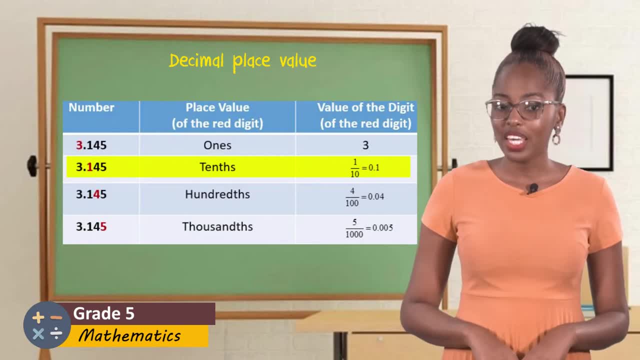 It can also be represented by the fraction one tenths. It can also be represented by a decimal that is 0.1. 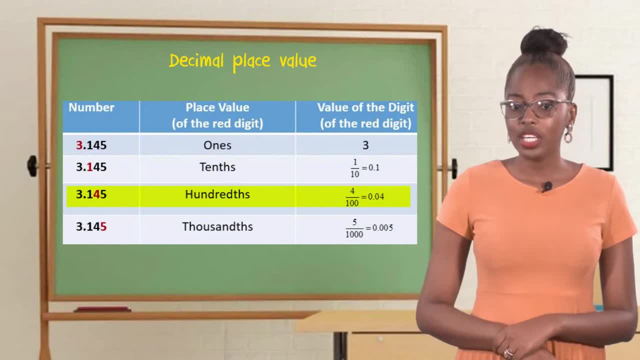 The place value of the numeral 4 is in the hundreds place value. That place value can be represented as a fraction where we put 4 as a numerator and 100 as a denominator. 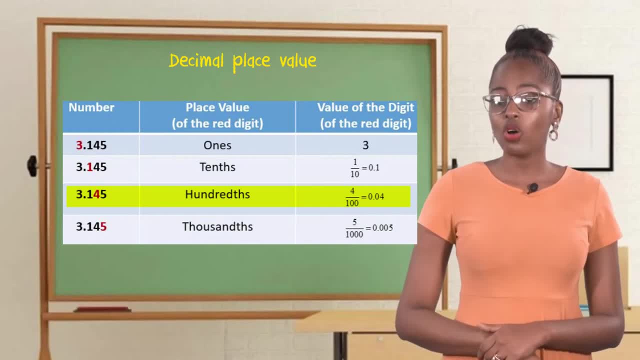 So that's 4.1. And we put 4 as a numerator and 100 as a denominator. So that's 4.1. And we put 4 as a denominator. So that's 4.1. And we put 4 as a denominator. So that's 4.1. And we put 4 as a denominator. But in the case of the number that comes up in the fourth place then we put 0 as a denominator so that's 0. Got it. Because it's showing that it answers like this. 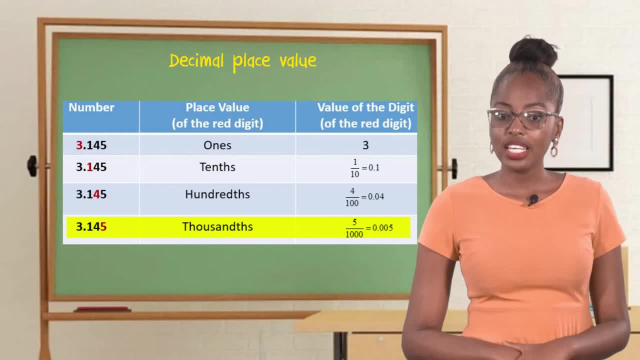 So this place value in a decimal is a decimal because in fact it's only a number which has count of zeros after it comes into a decimal number. 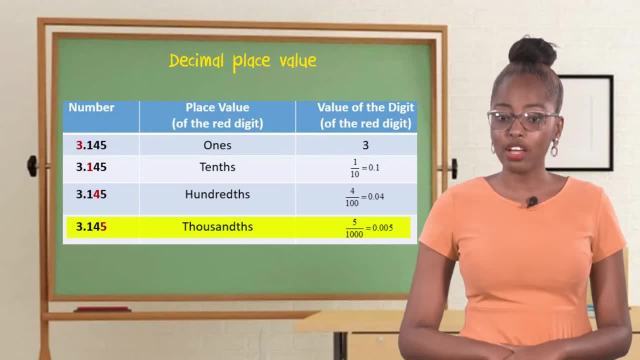 So for this it's a decimal to be represented by the 수�ensa in this one decimal фотографium we can also put the decimal into the decimal, so it can be represented by the sum of zeros in really simple form, right here, in the decimal right here. take Gutibbe discrete Galentine to find out which number this is the. 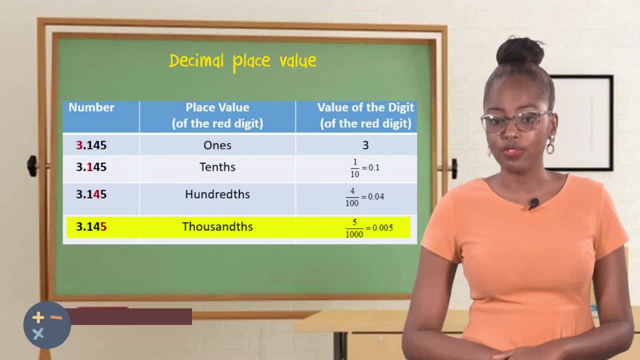 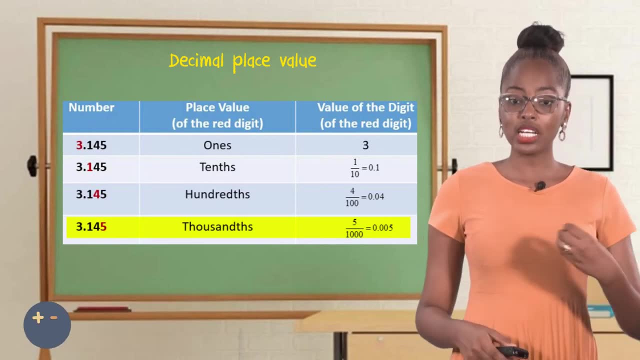 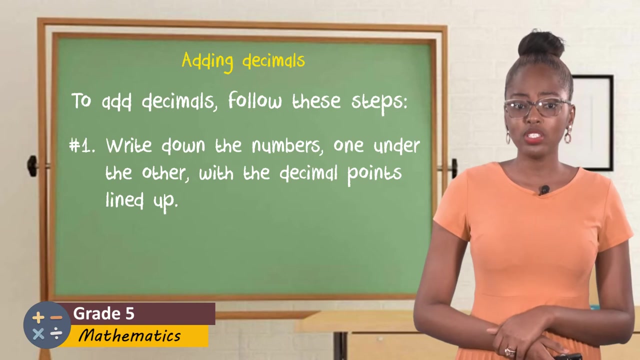 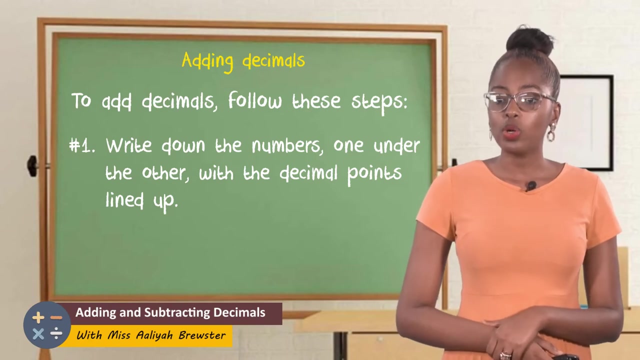 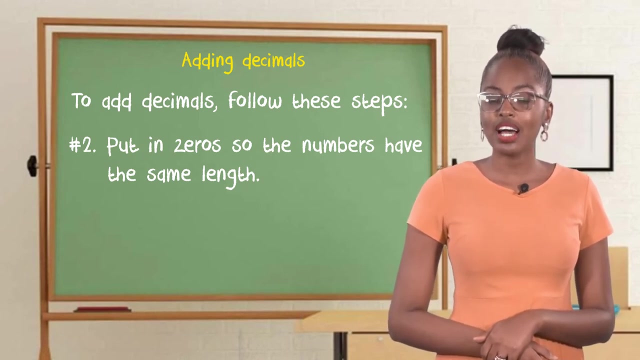 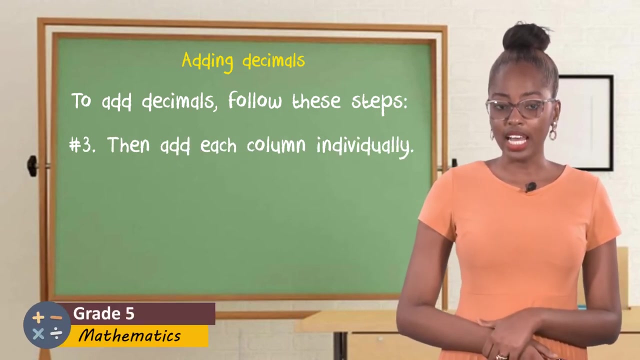 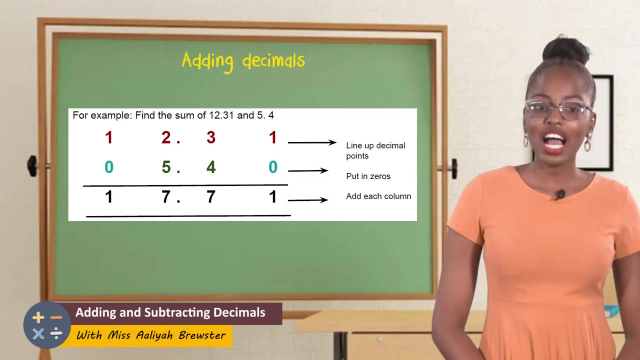 which is zero point zero zero five so what you need to grasp here boys and girls is that decimals can actually be expressed as a fraction and also it can be expressed as a decimal adding decimals to add decimals follow these steps number one write down the numbers one under the other with the decimal points lined up number two put in zeros so the numbers have the same length number three add each column individually and lastly remembering to put the decimal point in the answer let's say you're asked to find the sum of 12 and 31 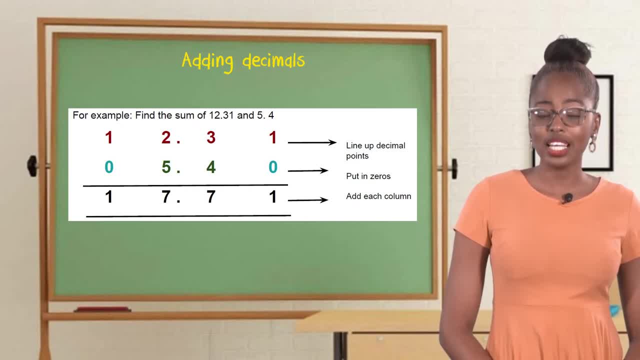 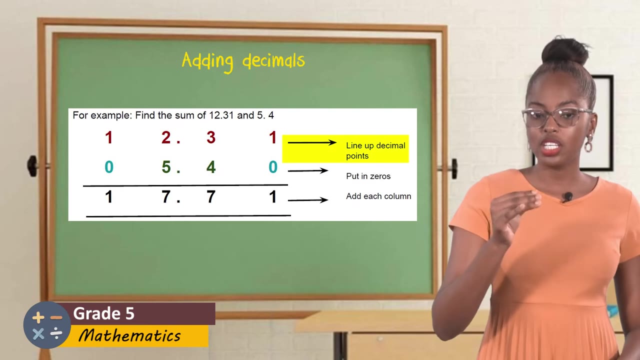 hundredths and five and four tenths how we'll do this we'll first start by setting the numbers having the decimals line up that simply means that you set the numbers in such a way that the points fall one under the other just as 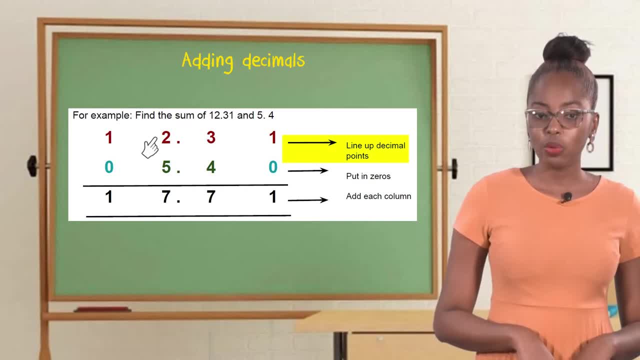 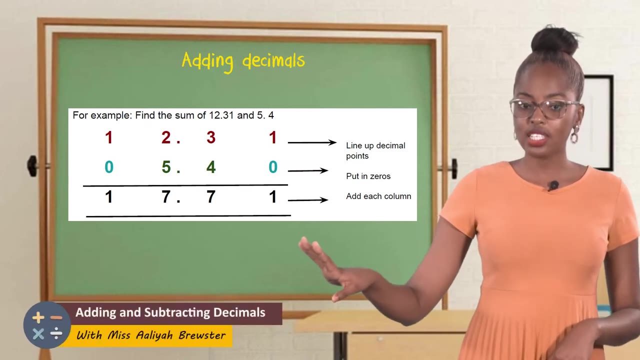 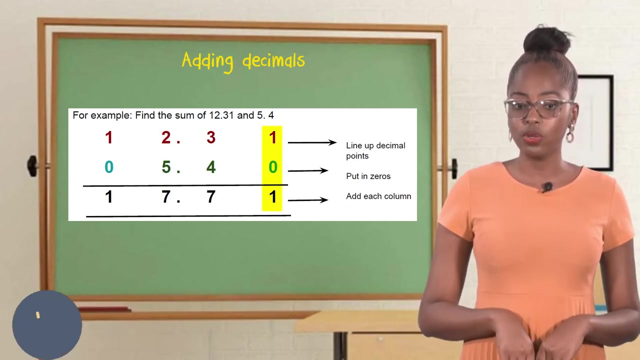 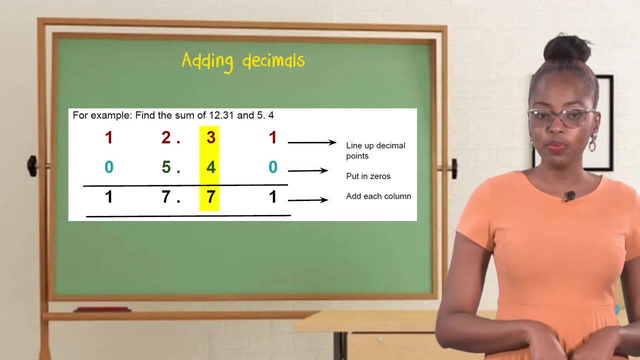 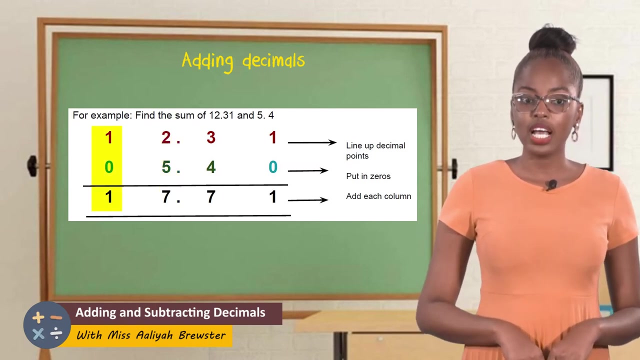 how you see it being depicted on the screen there we have point two and point five falling directly below each other so the next step is to add each column individually we'll start from the right and move to the left starting from the right we must first add one and zero that will give us one then the other column will add three and four that will give us seven then of course we write back the point and then we add two plus 5, we'll get 7. And then we add 1 plus 0, we'll get 1. Therefore, the answer for 12 and 3 to 100s 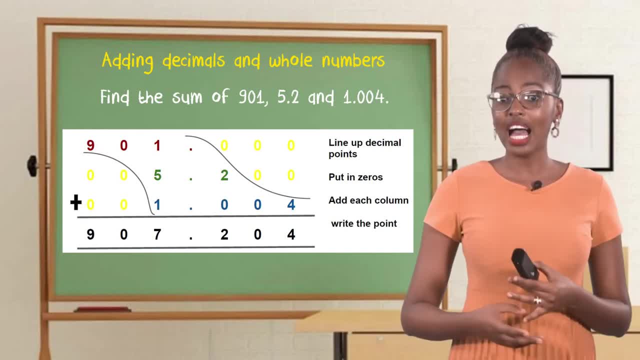 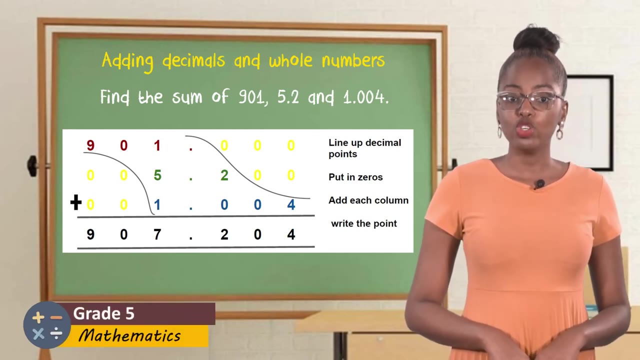 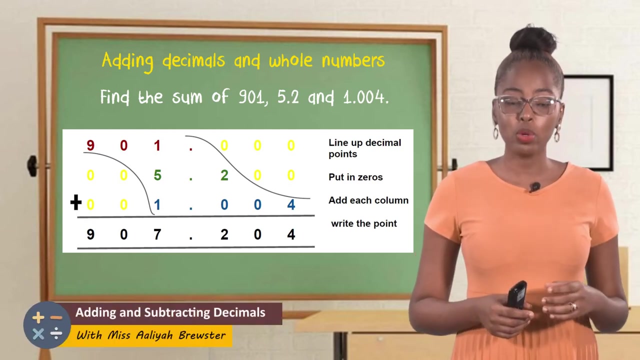 we'll examine how to add decimals and whole numbers. Suppose you're asked to find the sum of 901 plus 5 and 2 tenths and 1 and 4 thousandths. What you have to do, you remember that whole numbers always have a point at the back. We don't always include that point when we're writing whole numbers. However, whole numbers always have a point at the back. 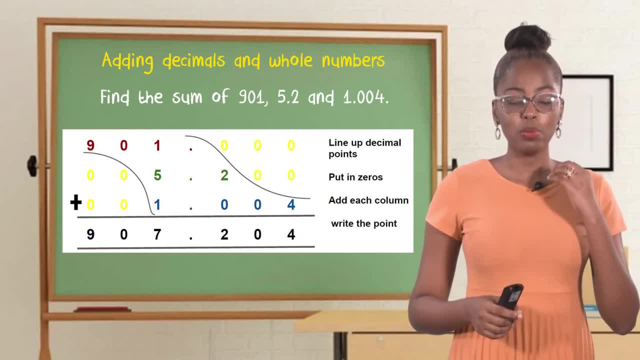 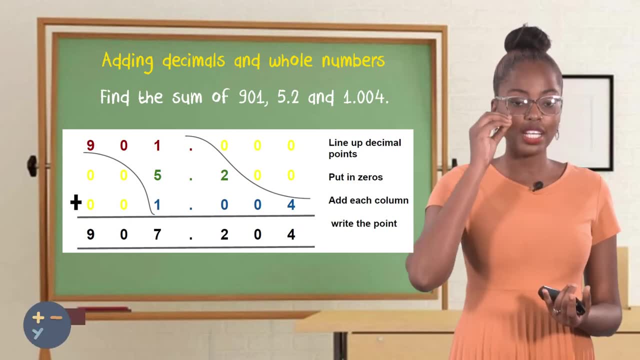 Therefore, when we're setting up our problem, we make sure to add the point at the back of the whole number and then have every other number with a point lined up exactly below that number. 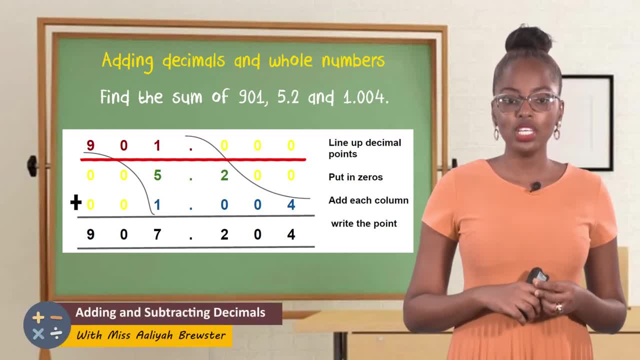 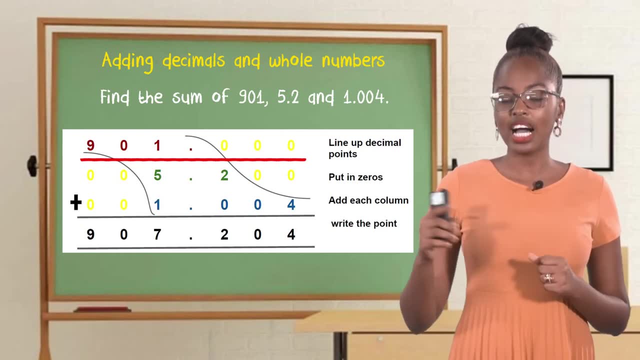 Look at the example on the screen. There you would see 901.000. Why did I put those three zeros at the end there? The reason being is so that you can see that the number is 901.000. Why did I put those three zeros at the end there? The reason being is so that you can see that the number is 901.000. Why did I put those three zeros at the end there? The reason being is so that you can see that the sum, 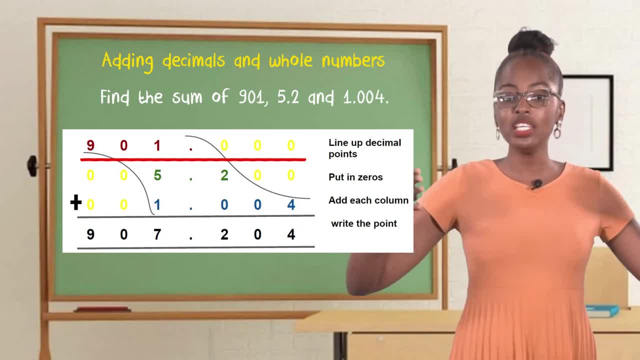 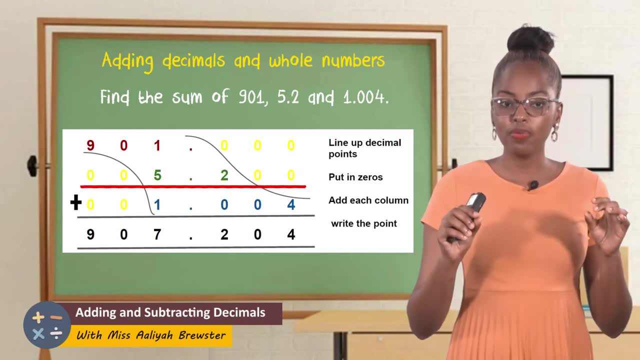 all of the the numerals will have the same length, so it will be easier for you to add and not get too confused, right? The other number 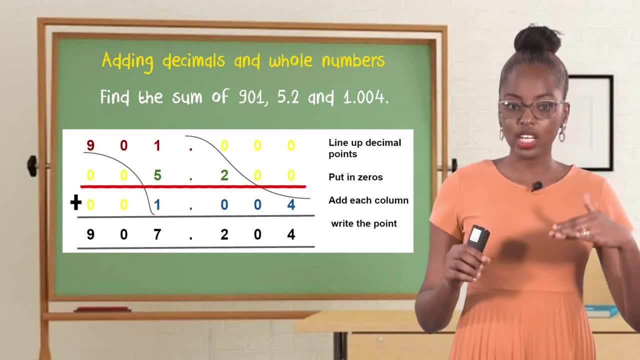 is 5 and 2 tenths, so again we put a point directly under the first point and we have five on the left side and two on the right side 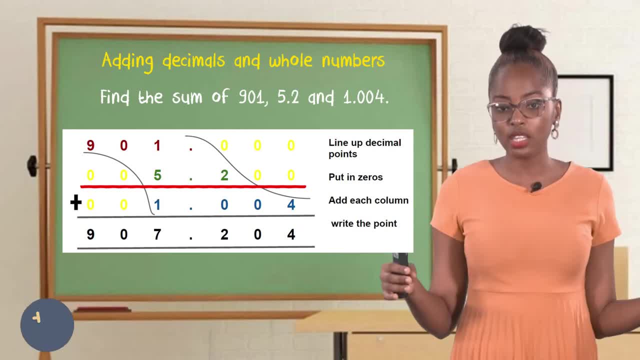 and we included some zeros in front and behind that number to make it the same length. 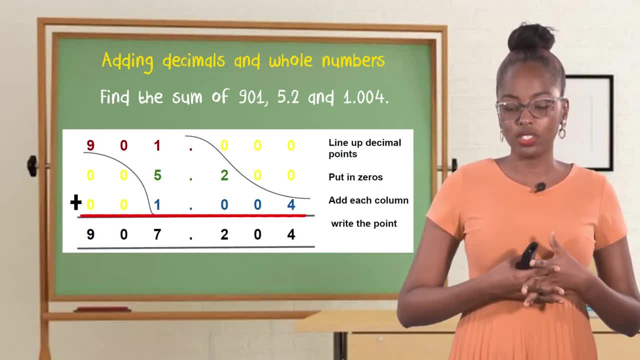 The last number there is 1 and 4 thousandths. 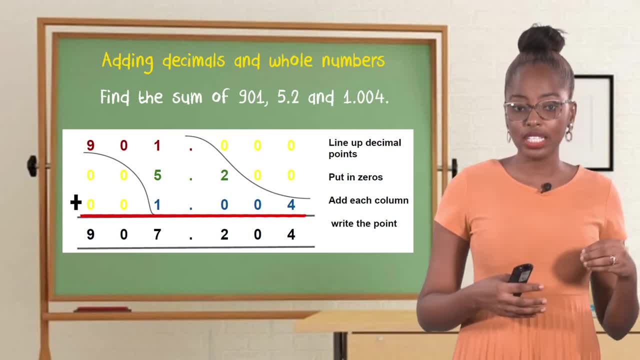 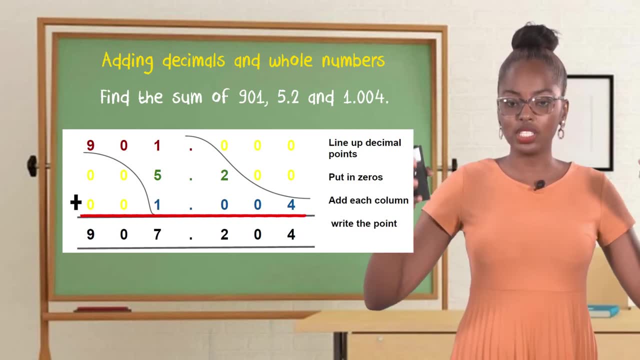 We included a point directly under the second point again. And then we added some zeros to make the number lying up in the same length. 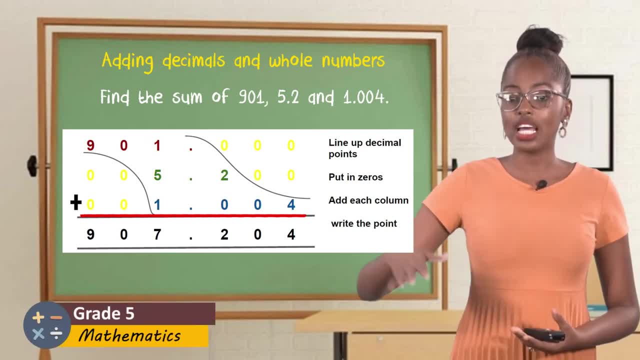 Now we can add each column. Again, we're starting from the right and we're moving to the left. Let's start from the right. 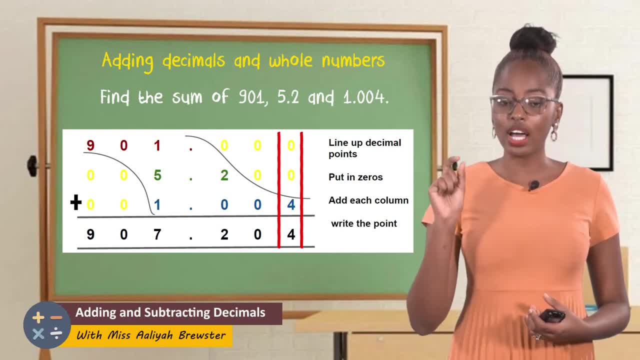 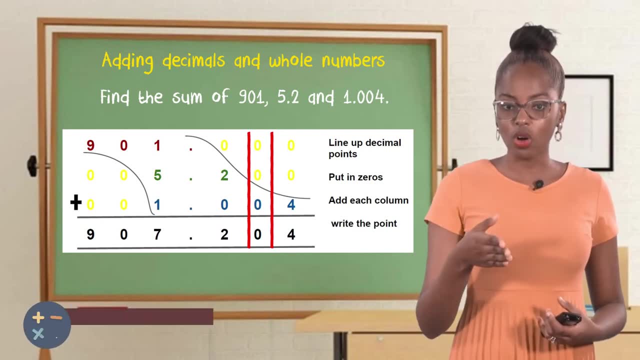 That first column there, we have 0, 0 and 4. So we add 0 plus 0 plus 4 will give us 4. The second column, we have 0 plus 0 plus 0 will give us 0. 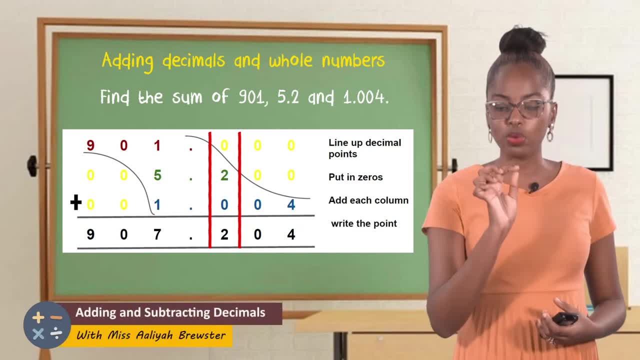 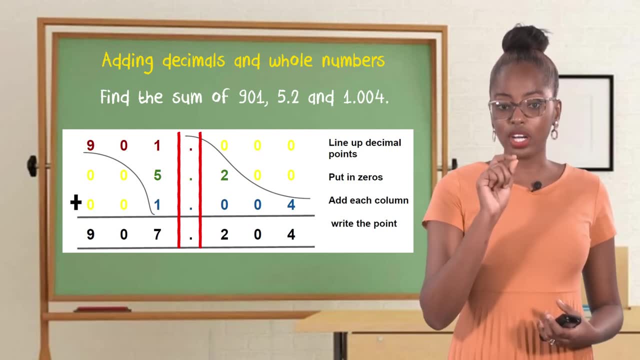 And the third column, we have 0 plus 2 plus 0 will give us 2. And then of course we write the point back into our answer. 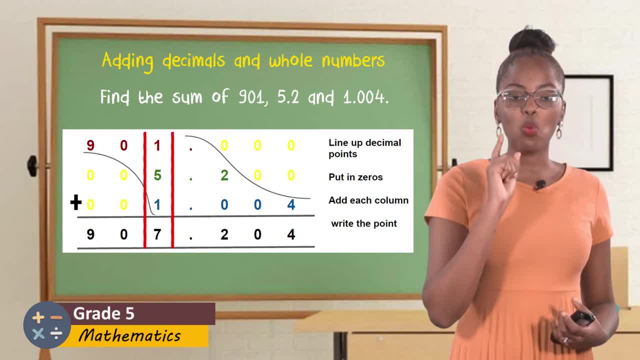 And then we move on to the fourth column. We have to add 1 plus 5 plus 1. That will equal... That will equal to 7. 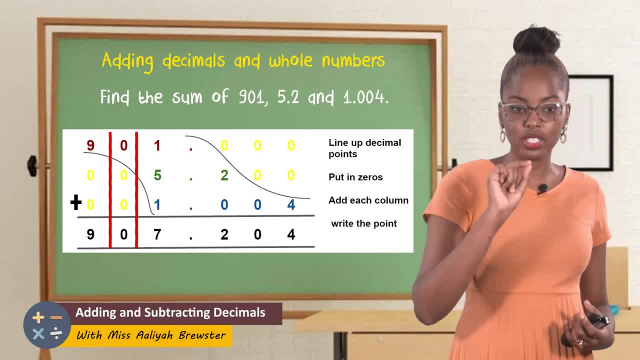 Then we'll add the second column which is 0 plus 0 plus 0. That will give us 0. 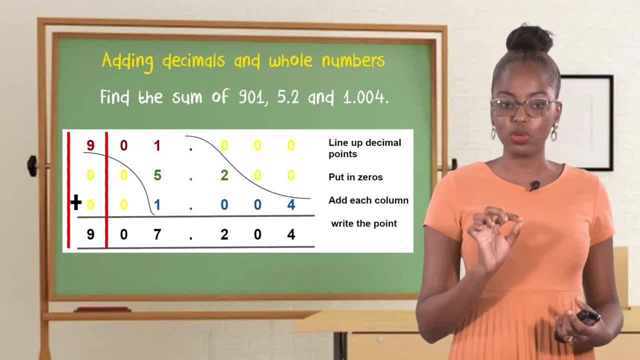 And then we add the last column which is 9 plus 0 plus 0 which will give us 9. 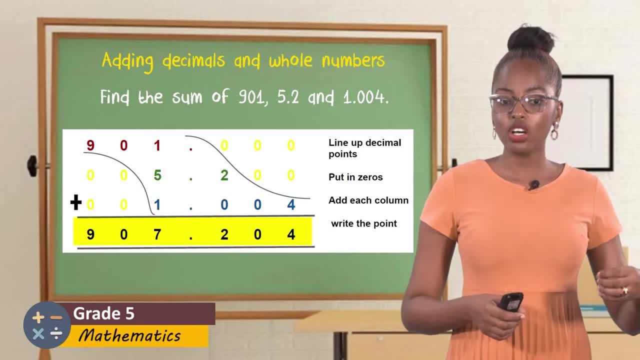 Therefore, the solution to this problem would be 907.204 thousandths. That would be the answer. 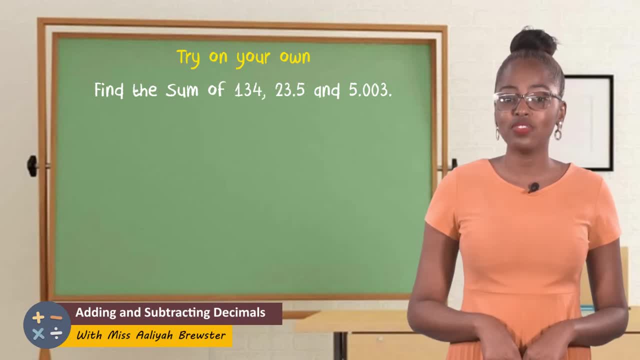 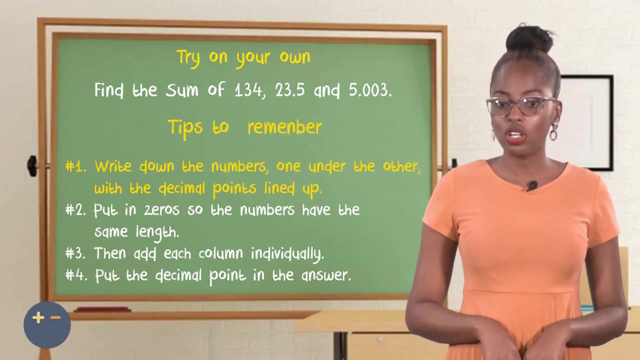 Okay boys and girls, now it's time for you to try an activity on your own. Find the sum of... 134, 23 and 5 tenths and 5 and 3 thousandths. Remember, write down the numbers one under the other with the decimal points lined up. Put zeros in so the numbers have the same length. Then you add each column individually and remember to include the decimal point in your answer. 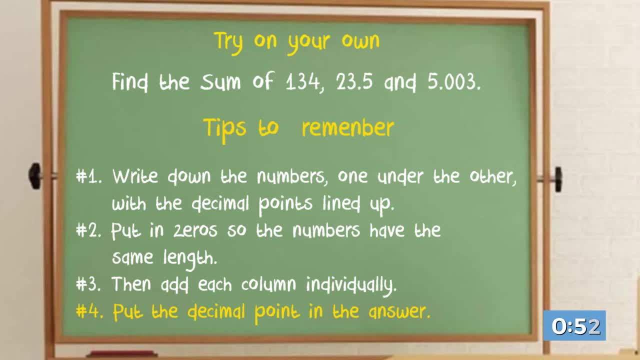 I want to make sure we give the spell section credit siendo 6% of all the cases 6. 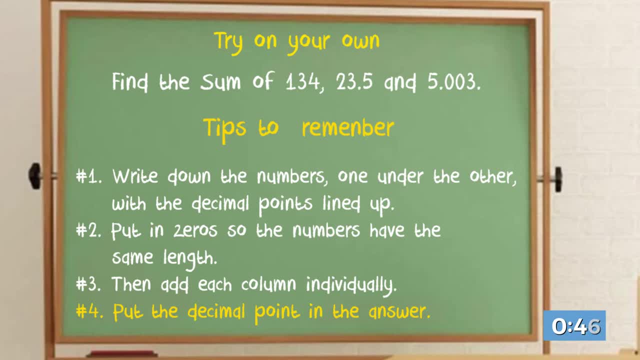 Let's write that down and let's pass our class criteria to everything else. 8 comprehension power is equal to 2. 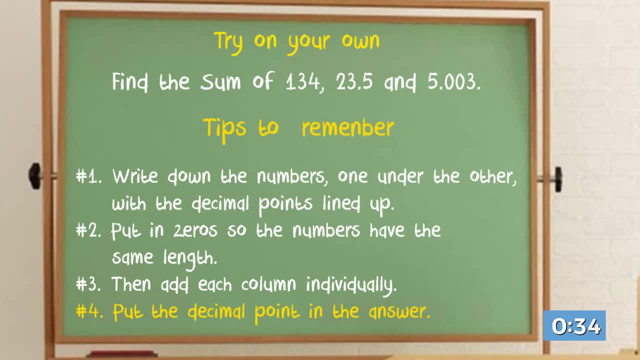 We have the answer to 4 questions. Yeah, we haveก resolving all this. Yeah. 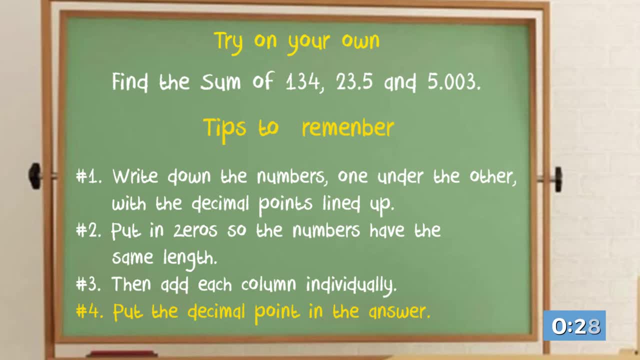 If you would please repeat 9,988 hours. Okay. Thank you. That's all. Thank you. Thank you. Bye. 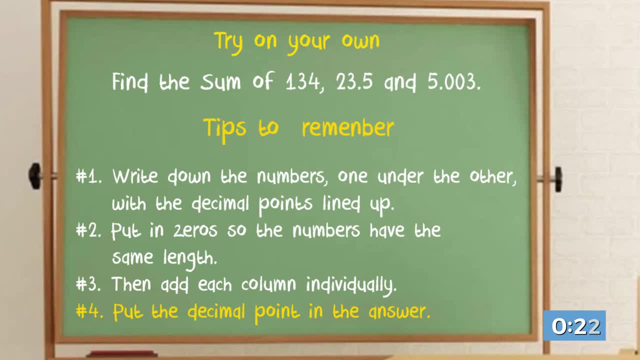 Did you get it correct? Let's go through. 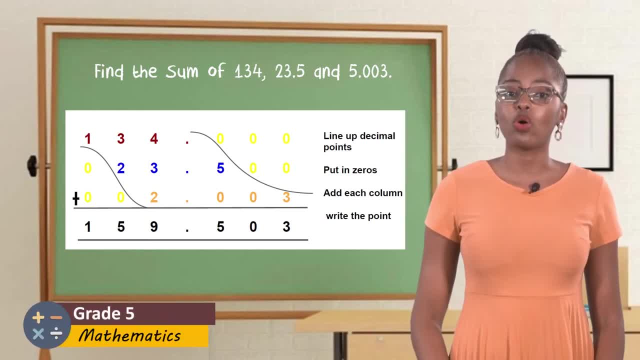 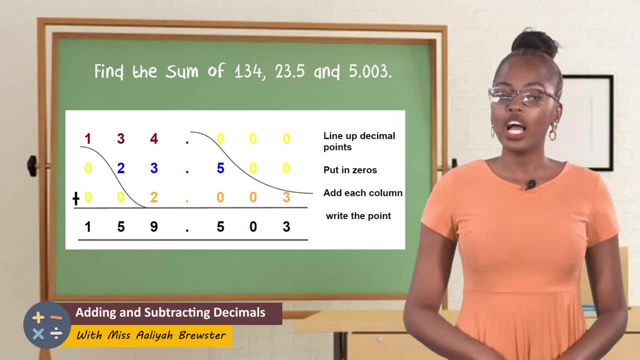 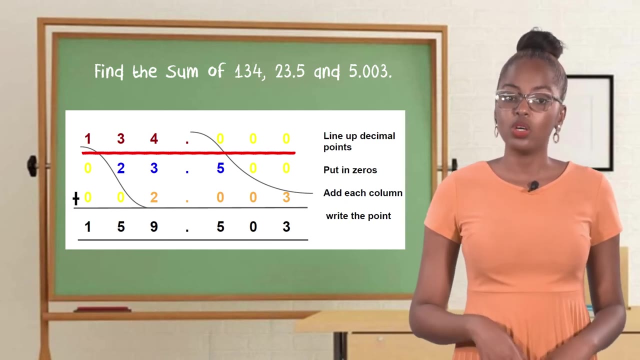 We were tasked in finding the sum of 134, 23 and 5 tenths, and 2 and 3 thousandths. We begin by first lining up the decimal points. We said that a whole number always has a point at the back. Even though it may not be written in, it is an understood rule that every whole number has a point at the back. 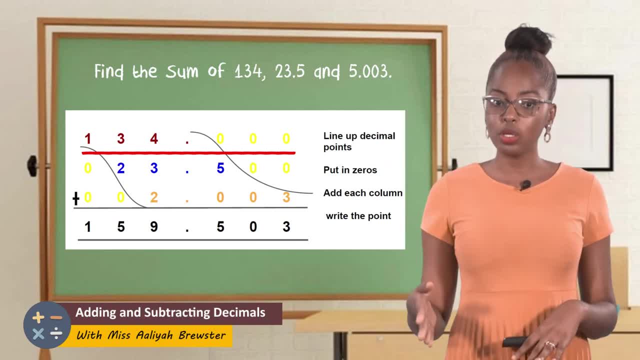 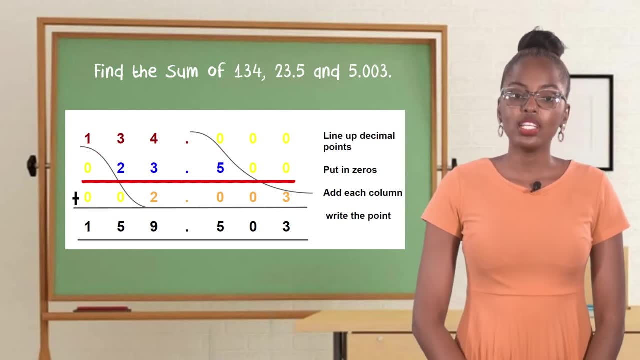 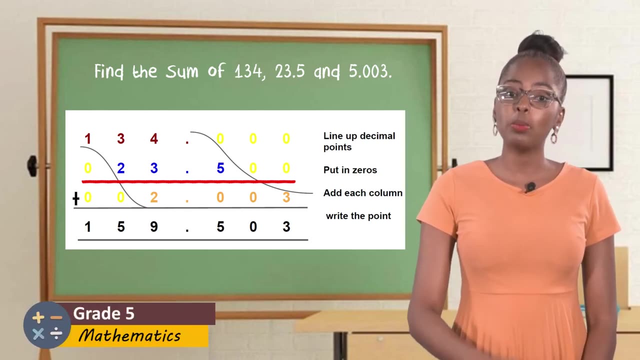 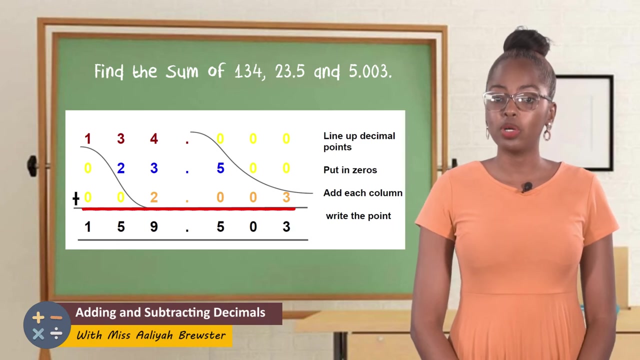 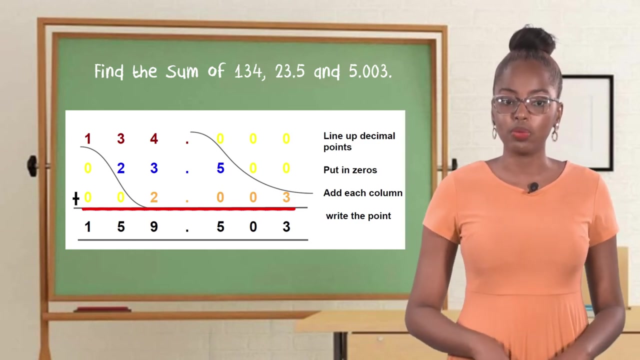 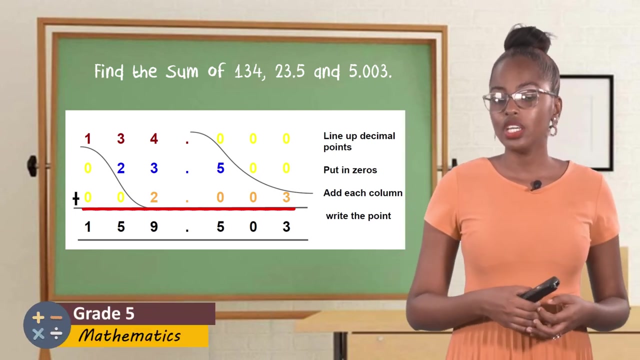 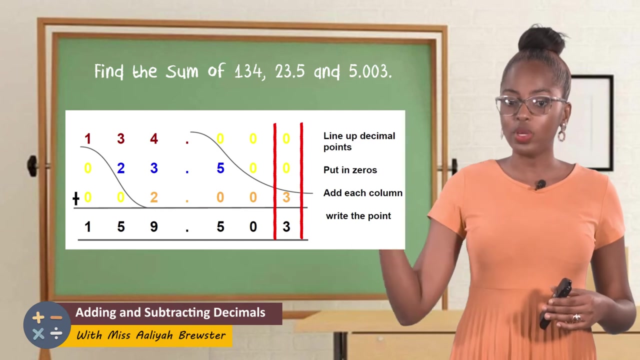 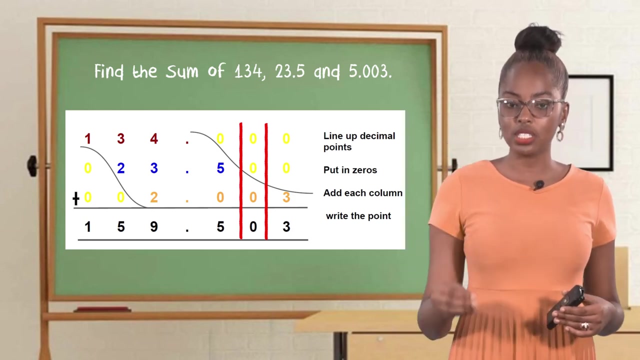 Therefore, we write the whole number, we put the point at the back, and then we add zeros to make it the same length as the others. Then we'll set the number 23 and 5 tenths just below 134, with the point lined up exactly under the first number. Then we'll set up the number 2 and 3 thousandths, with the point lined up exactly below the first number. Then, of course, we'll add the zeros to make them all the same length, so it's easier for us to add. Starting from the right and moving to the left, we begin to add. The first column from the right, we add 0 plus 0 plus 3, we'll get 3. Then the second column, we'll add 0 plus 0 plus 0, we'll get 0, of course. And then the third column, we add 0 plus 5 plus 0, we'll get 5. And then, of course, we write the point back, that is very important. 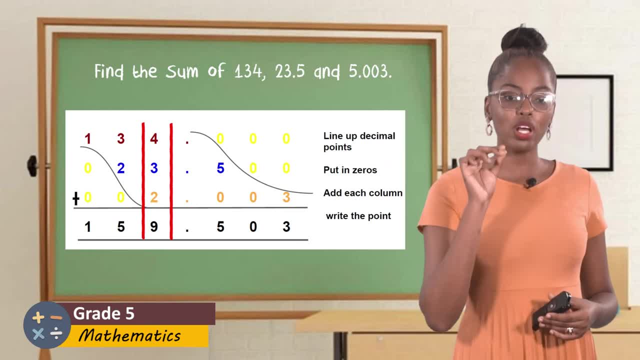 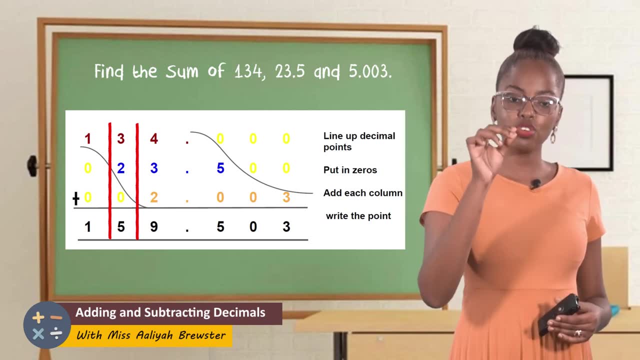 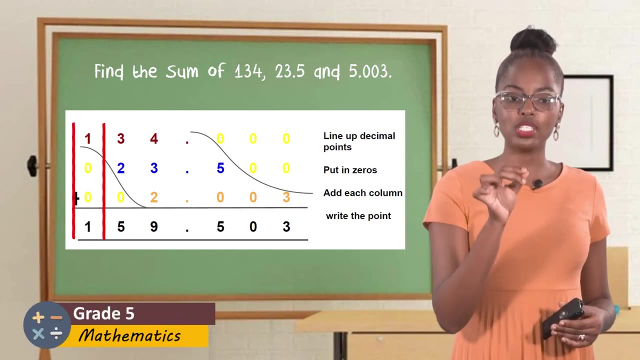 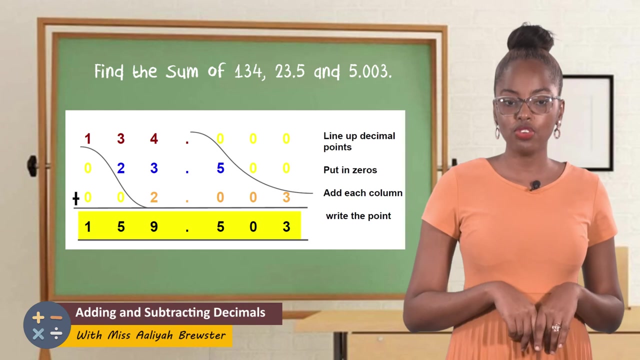 And then we'll move on to the fourth column, we add 4 plus 3 plus 2, and that will give us 9. And then we add the fifth column, which is 3 plus 2 plus 0, that will give us 5. And then we add the last column, which is 1 plus 0 plus 0, and that will give us 1. Now that we have our answer, we know that the solution is 159. 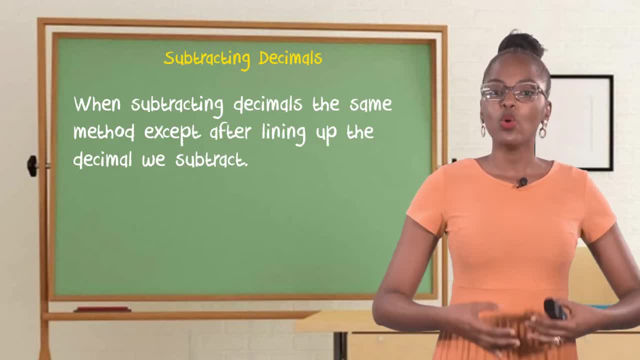 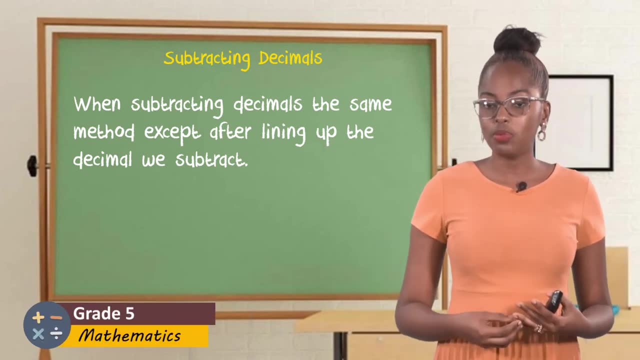 Now, boys and girls, we'll move on to subtracting decimals. When subtracting decimals, the same method is applied as adding decimals. After we finish lining up the decimal points, we subtract instead of add. For example, suppose we're asked to solve this problem. 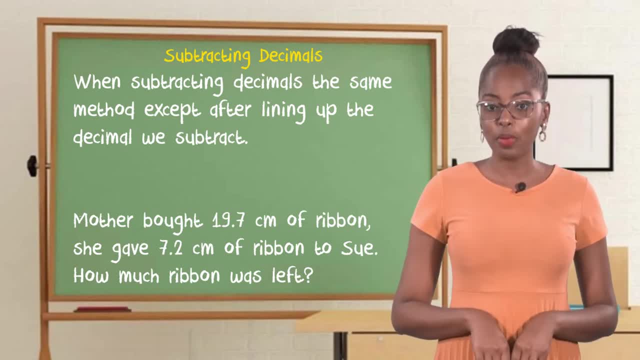 Mother bought 19 and 7 tenths cm of ribbon, and she gave 7 and 2 tenths cm of ribbon to Sue. How much ribbon was left? 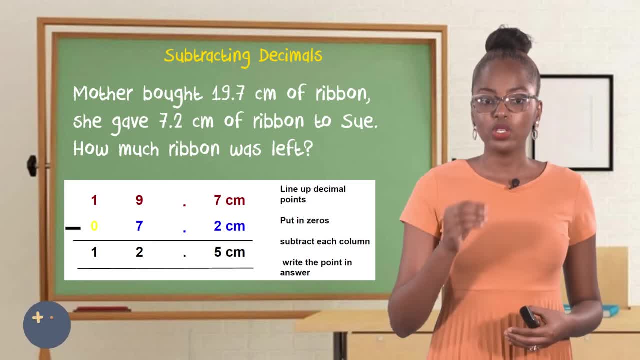 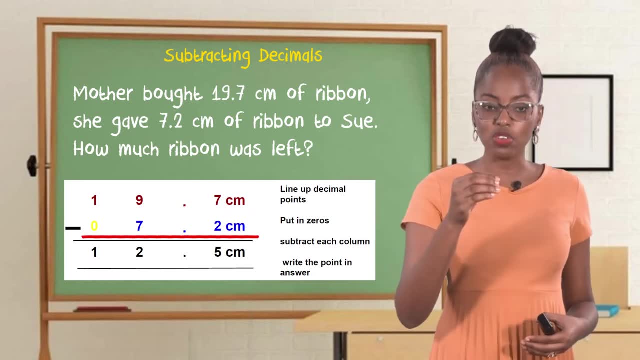 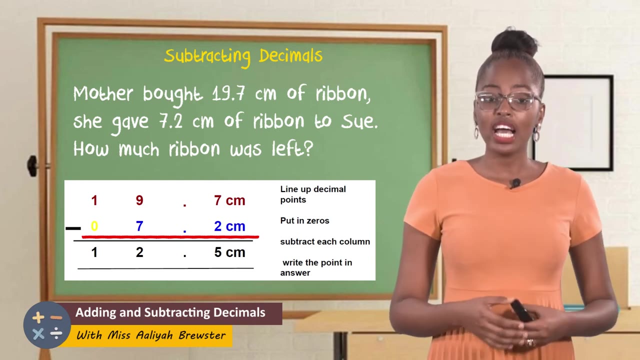 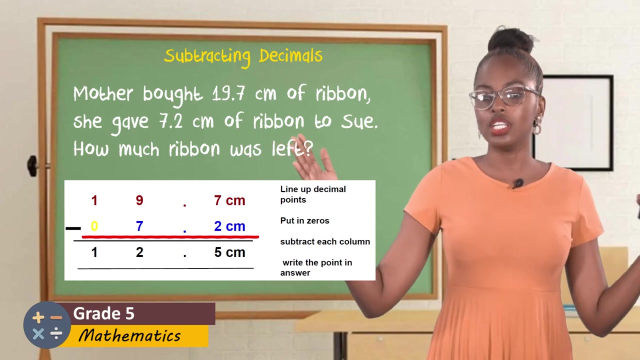 Okay, we begin by lining up the decimal points. So we start by setting up 19 and 7 tenths cm, and then just below that, we write 7 and 2 tenths cm, with the points falling directly below each other. And then I add in a 0 there to make the two numbers the same length. Now we can add from the right going to the left. We start. We start. 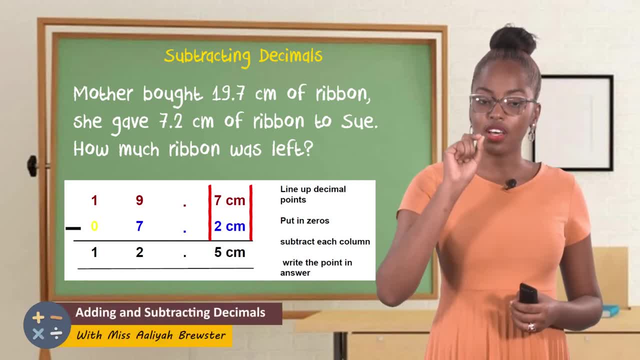 7 minus 2 will give us 5. 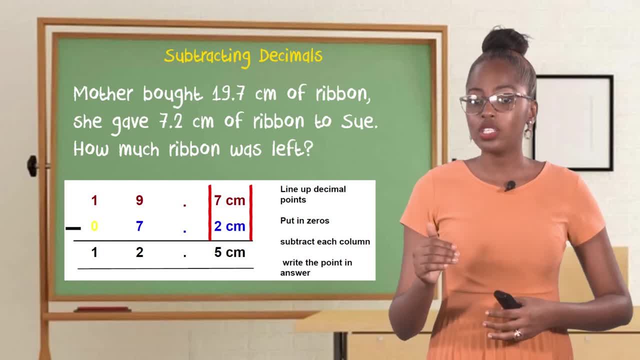 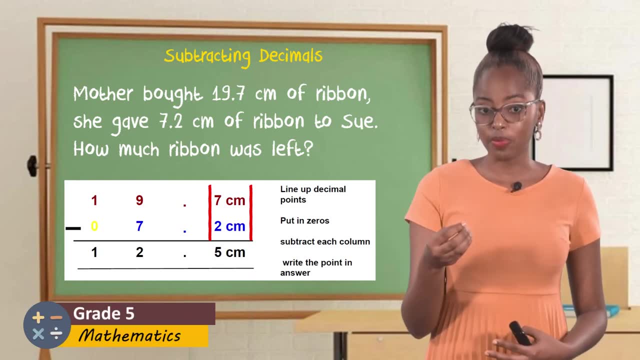 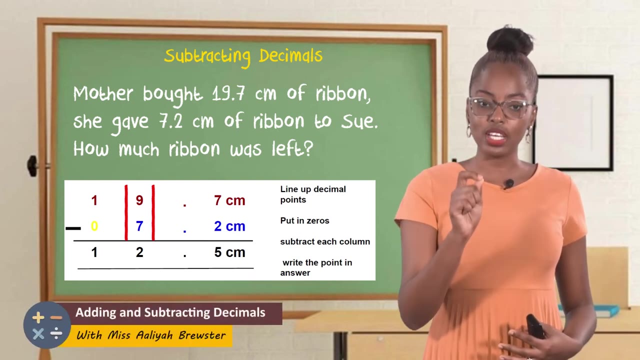 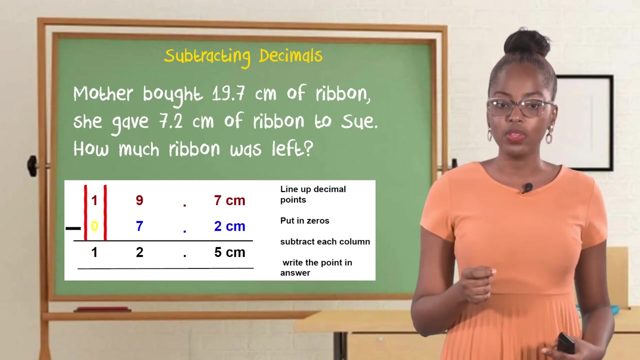 And if you notice there, I wrote back cm, because our answer should be written in the unit that we're calculating, and the unit here is cm, right? Then, of course, we write back the point, and then we move to the second column. We minus 9 from 7, and that answer would be 2. And then 1 minus 0 would, of course, be 1. Therefore, the answer would be 12 and 5 tenths cm. You can try this activity on your own. 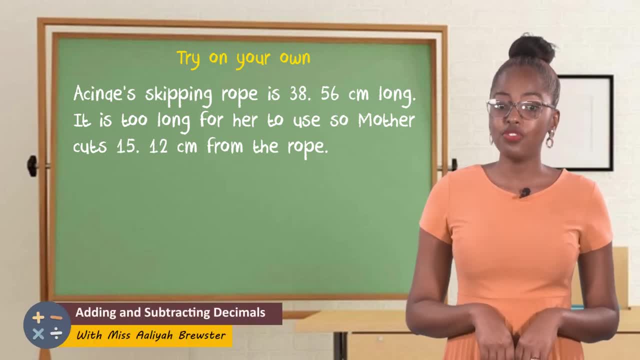 Asyna's skipping rope is 38 and 56 hundredths cm long. 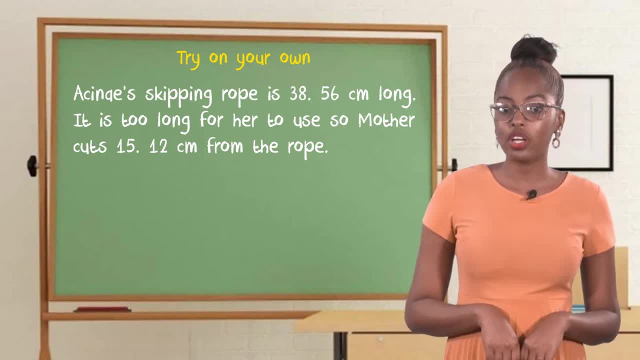 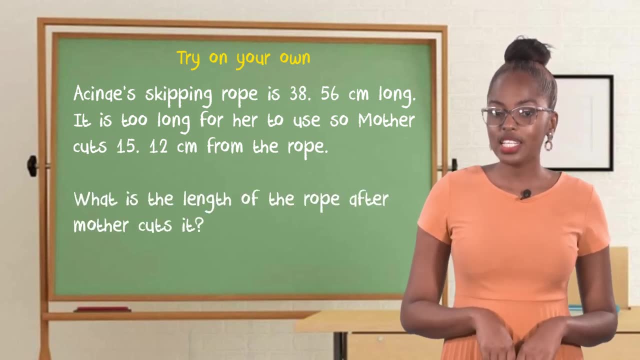 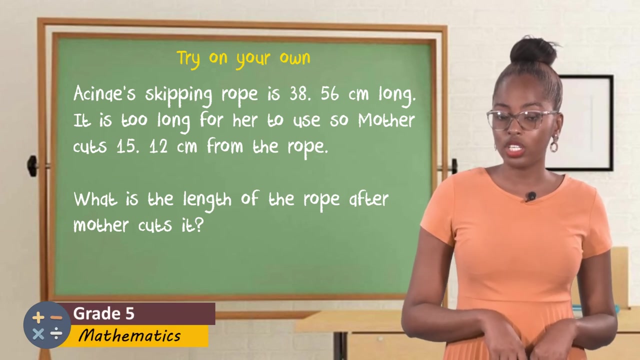 It is too long for her to use, so mother cuts 15 and 12 hundredths cm from the rope. What is the length of the rope after mother cuts it? Remember? You write down the numbers, one under the other, with the decimal points lined up. Put in 0 so the numbers have the same length. Then you subtract each column individually. And remember to include a decimal point in your answer. 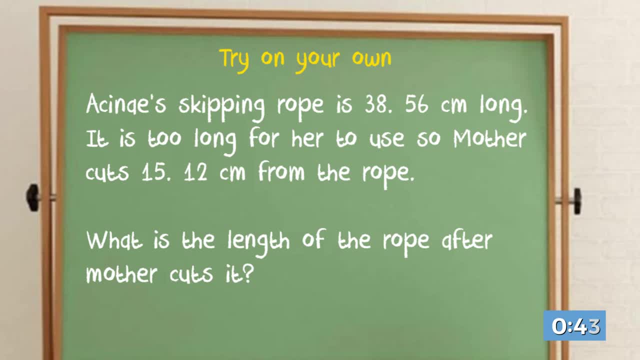 We write down the number of the first and second terms. Now we're going to take a look at the number of the first and second terms. You can write down the number of the first and second terms. In this case, it's 1. Not a decimal! Is it a decimal? You're wrong. Sometimes there are two. It's not a decimal. It's a method. 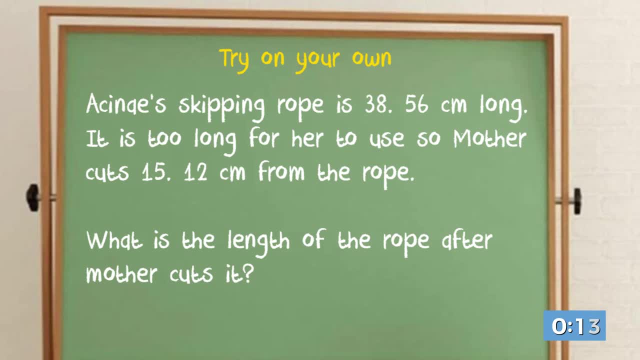 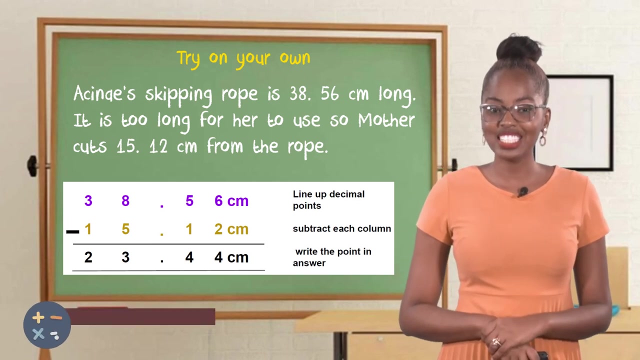 Did you get it correct? Let's check. 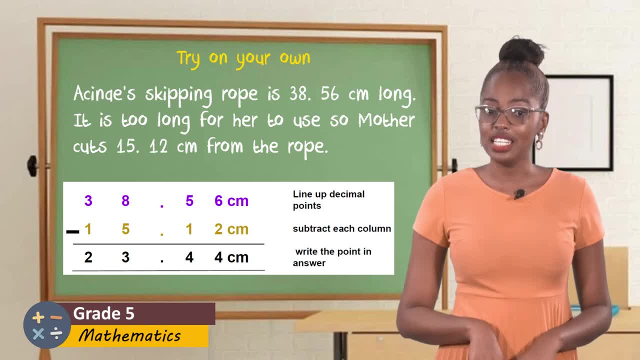 The problem we were asked to solve is ACNA skipping rope is 38 and 56,000 cm long.